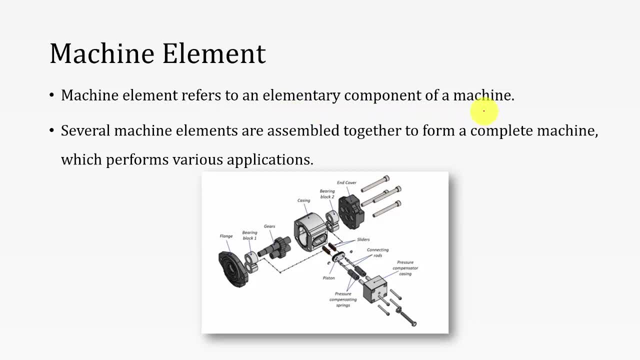 element refers to an elementary component of a machine. So this is the basic component of a machine, and several machine elements are assembled together to form a complete machine. So the machine performs various applications. So to perform the various applications there are many machine elements are assembled together to form a complete machine. So to perform. 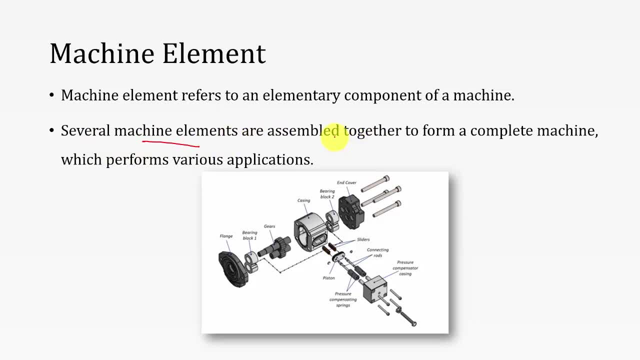 the various applications. there are. many machine elements are assembled together to form a complete machine. For example, you can see here: So here we have a gear, we have a casing, we have a bearing, then we have a flange, then we have some connecting rod. So all these 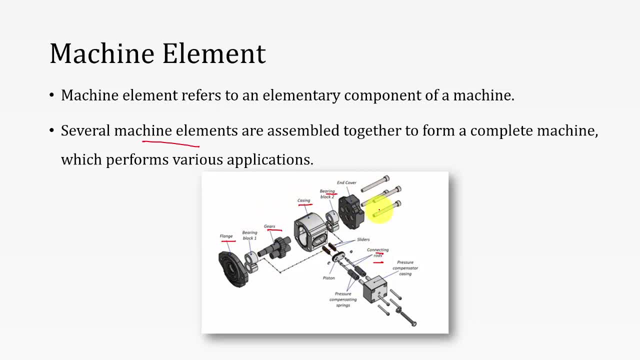 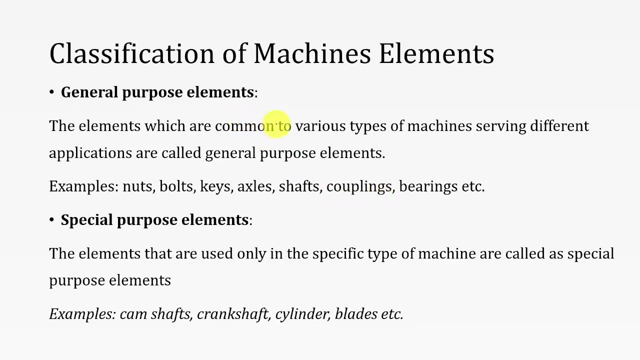 machine elements are connected, assembled together to form a complete machine. So the machine element is the basic part of a machine. There are two types of machine elements are there. The first one is general purpose element and the second one is special purpose element. 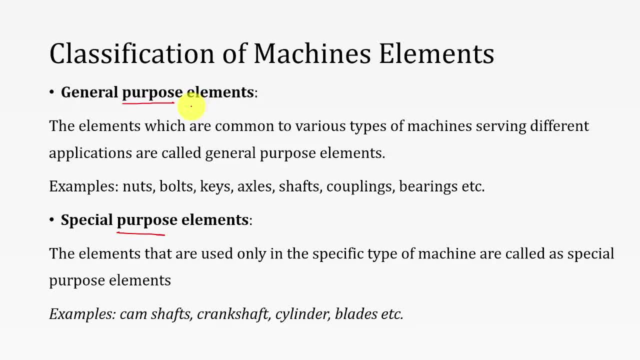 These general purpose machine elements we use to carry out various applications, So these are all common. So a single bolt can be used for many applications, A single nut can be used for any application and, like wise, we have keys, we have shafts. 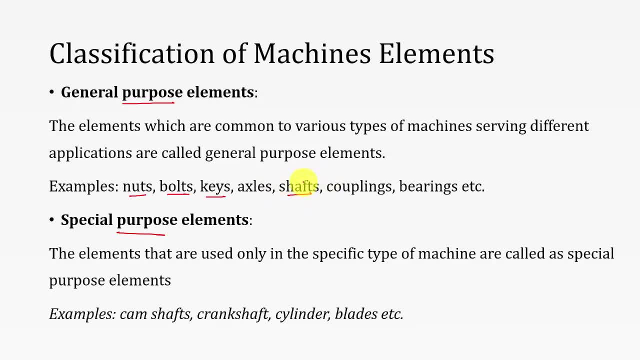 So shafts will be used for various power transmission applications. So this general purpose elements do not depends on the applications. Then the second one is special purpose element elements. So this special purpose machine elements are used to perform only the special applications. For example, here we have the example as camshaft, So this camshaft is 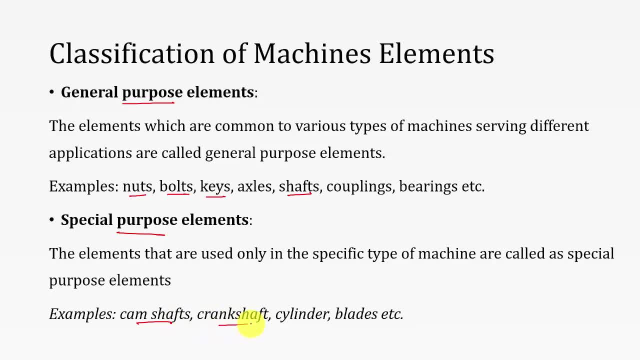 only used for cam. Similarly, the crankshaft is only used for crank. Similarly we have blades and we have cylinders. So these kind of machine elements are only used for some specific application, to perform some specific operations. So that is the difference between. 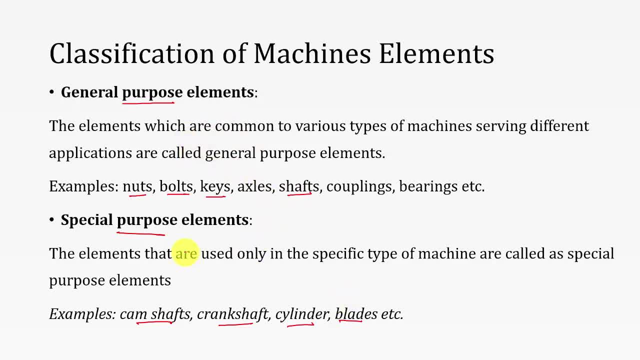 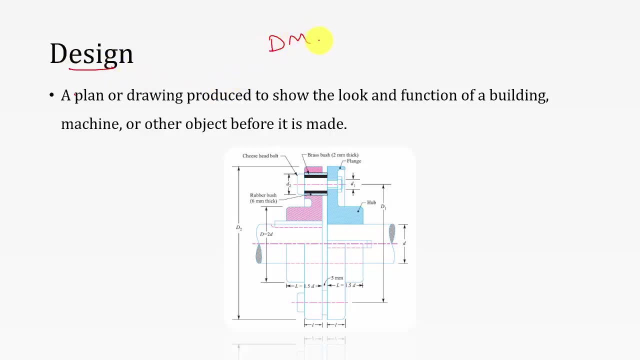 general purpose element and the special purpose element. So in this subject we are going to design both the general purpose element and a few of the special purpose elements. Then what is design? So I have splitted the design of machine elements into two. That 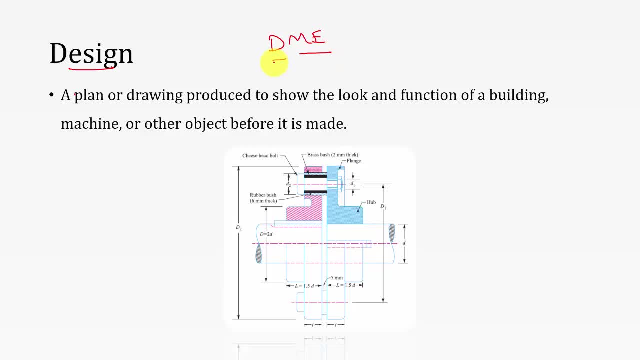 is the machine element and the design. So we have seen What is machine element. Now, what is design? So design is actually the language of an engineer. So it is a plan or a drawing produced to show the look and the function of a building. 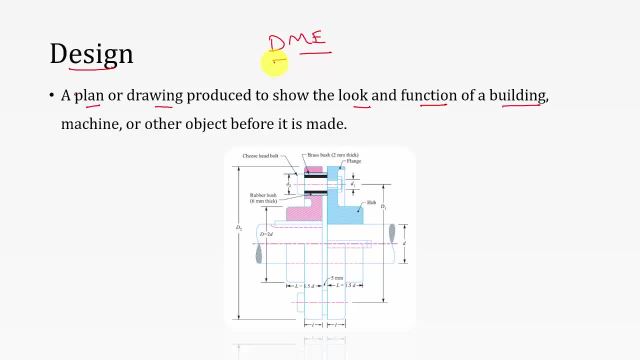 So if you are a civil engineer, then your design refers to a building. If you are a mechanical engineer, then it is a machine design. So it is a plan or a drawing. It is produced to show how it looks and the functions, along with the dimensions. So here you can. 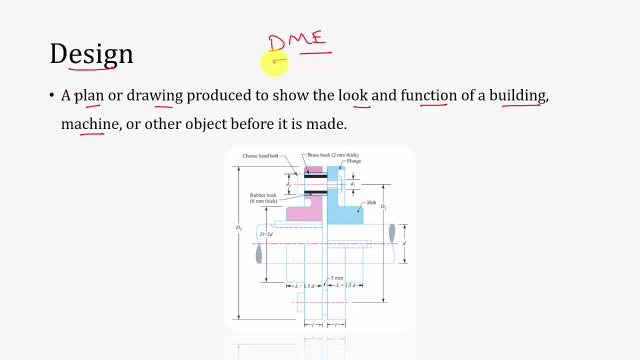 see that. So this is how A coupling looks like, And here I have also mentioned the dimensions. So this is a complete design. So a design engineer can prepare a drawing and he can give it to the production department. So the design is the communication between a design engineer and the production. 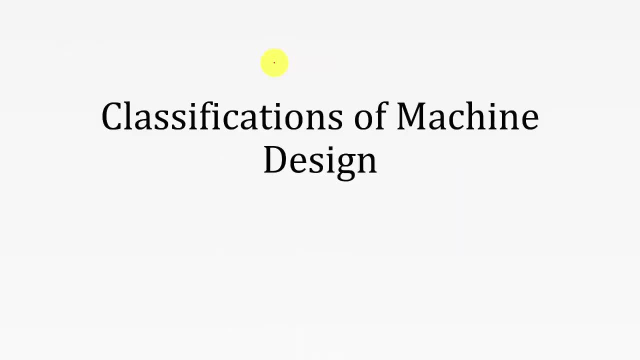 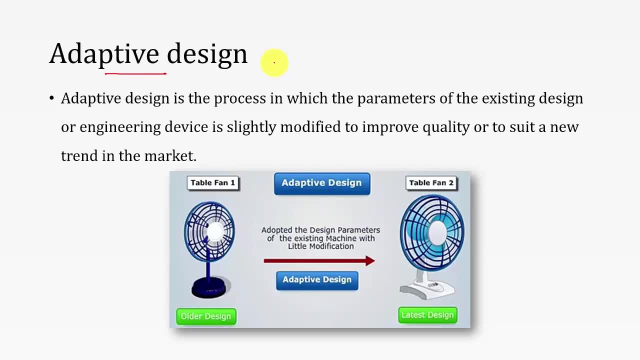 department, Then the classifications of machine design. So first of all the machine design is classified into three. The first one is adaptive design. So adaptive design means we are not going to do any modifications with the working principle of the machine. We are going to do some small parameter changes. That is, we are going to 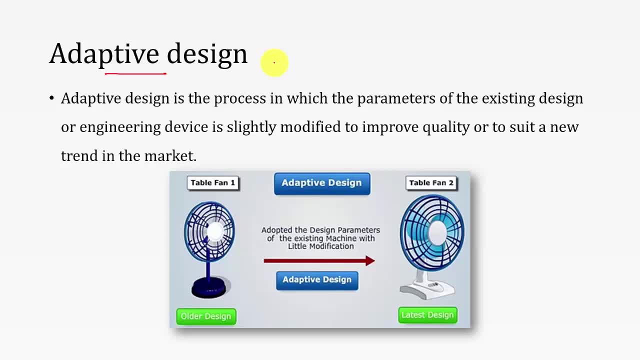 add some of the additional features with the basic machine, For example, you can see that. So here it is a table fan. The function of a table fan is to provide fresh air. So here the blades has to rotate. So that is the basic function. So here I have changed the. 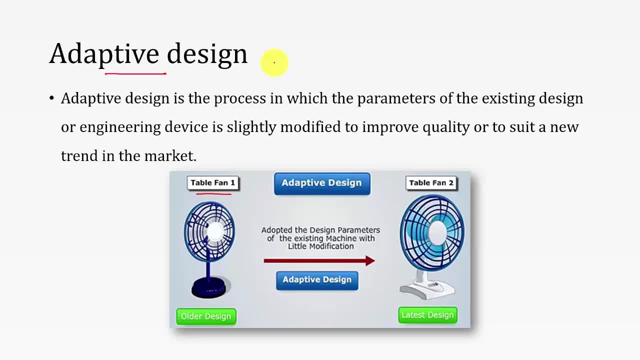 design of the table fan into an advanced one. So this is an olden days table fan. Now we have a new and weightless table fan. Ok, So here, In the first design the blades are made of steel, But here it is made of plastic. So 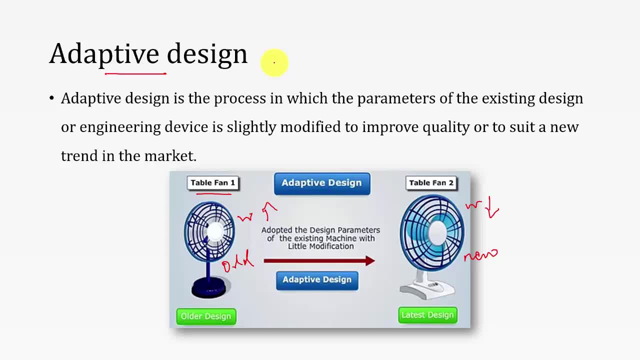 here the weight is high, Here the weight is minimal. So this is called adaptive design. We are not going to do any modifications, But still we are going to do only dangerouschecks. Ok, So this is adaptive design. design, This is one element only. This is called a welcomed movement. 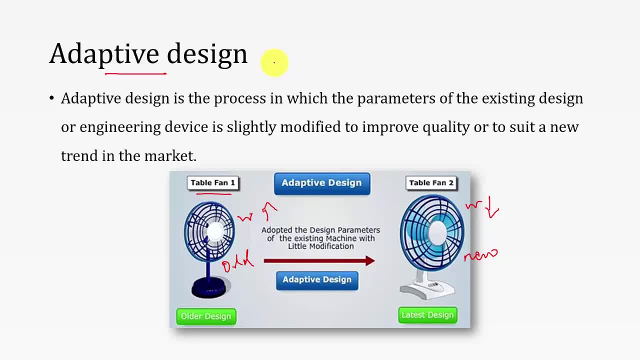 modification with the working principle of the design. but we are going to do some addition. we are going to add some additional features or we are going to do some modifications. so here, for example, here we have reduced the weight. so by reducing the weight of the blades we can get energy efficiency. so likewise. 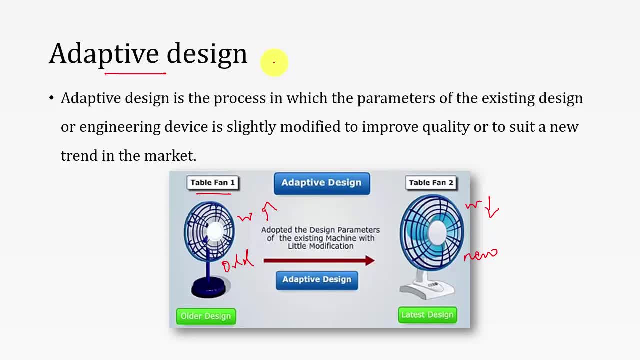 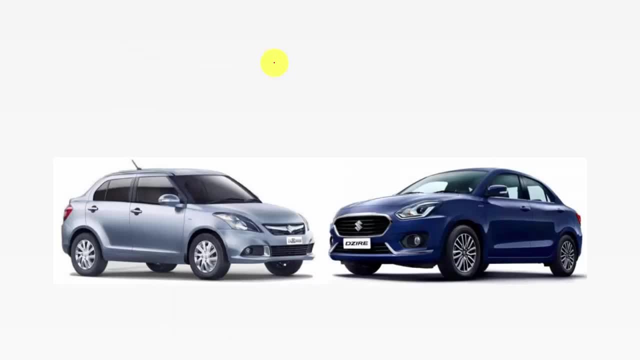 we can add some of the new features, so that is called as adaptive design. so this is another one example of adaptive design. so this is a shift desire. so this is old model and this is new model. so all the specifications are almost equal. only thing is they have modified some of the design so that it can attract the 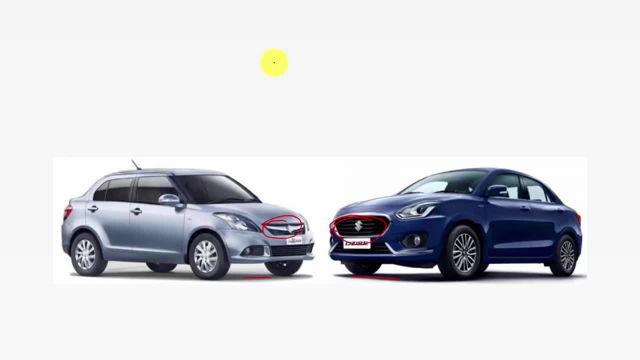 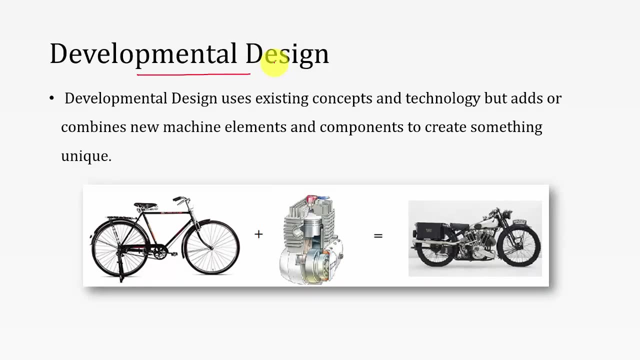 people. so that is the basic reason for adaptive design. next one is developmental design. so here we are going to add some new concept or new technology so that we will change the working principle. okay, so the basic working principle of the mission will be changed. so here mostly. 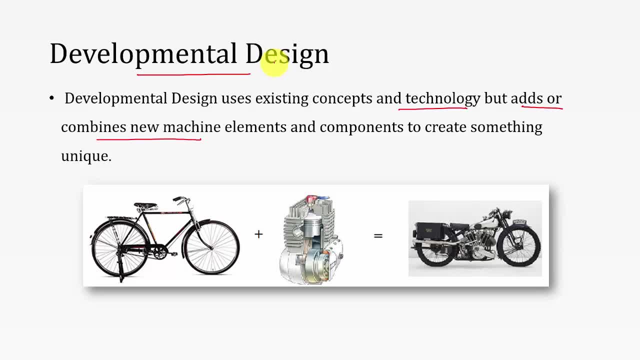 we will add or combine two missions together to get a new mission. so here the engine is fitted with the cycle so that the basic function is modified, but the wheels, the hand bar and all those things are uniform. so here this is actually a development of the cycle. the bike is the development of a cycle. okay. 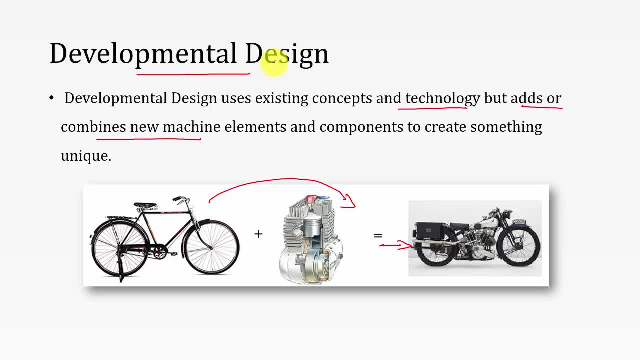 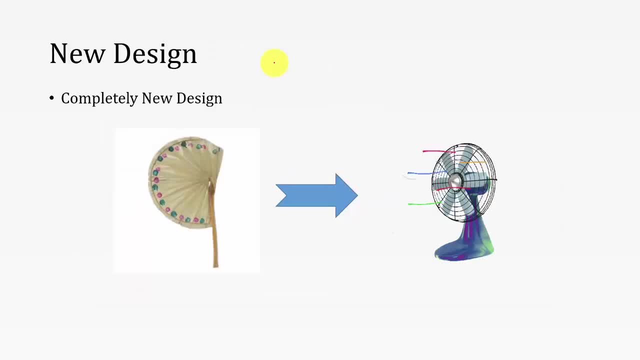 so this is called a cycle. so this is the development of a cycle, so this is called a developmental design. so we are developing something, we are adding a new technology, but here the basic operation will be changed. the last one is new design, so it's completely a new design. so there is no such components or there. 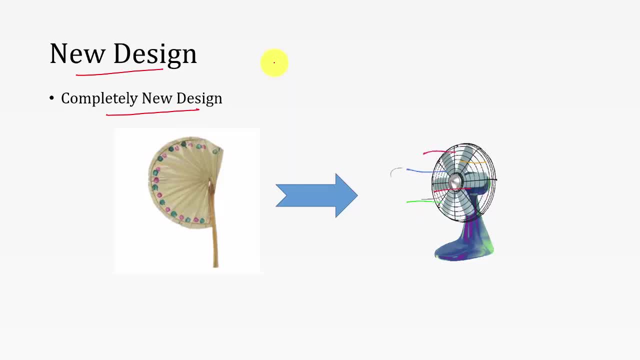 is no such mission exists in the previous. okay, so that is called as a complete new design. so here, assume that we don't have any fan. so now I am implementing a new fan, then it comes under a new design. so we don't have any cars in the universe. so if I implement a car, then it 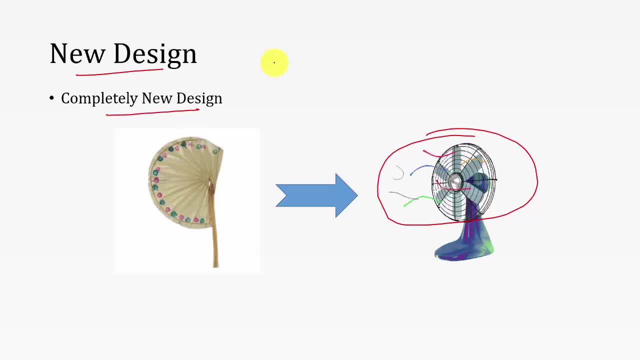 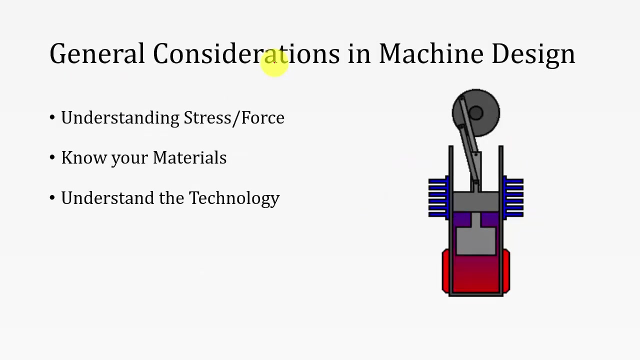 is comes under new design. so if you are designing a new mission, so for your project, maybe if you are designing a completely new mission to perform any new application, then it comes under new design. okay, so these are all the three classifications of mission: design, then the general considerations in mission. 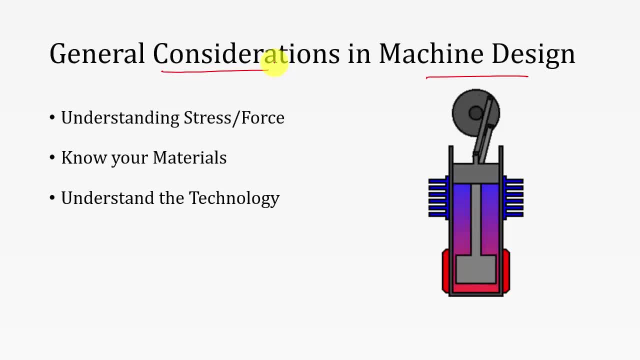 design. so three factors to be considered while designing any mission component. the first one is understanding the stress and the force. okay, so to avoid unwanted failures are two. so to design the mission, to cap, to carry the allowable loads, we have to calculate the type of load acting. so there are plenty of loads will be acting in a mission element. so 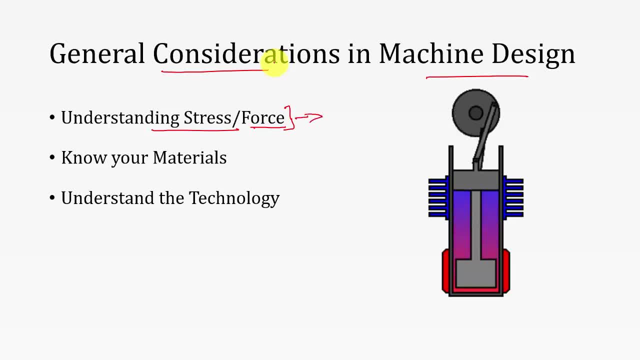 first up, we have to identify the type of force is acting on the mission. so once after identifying the nature of the force, then we can calculate the amount of stress. ok, so the amount of stress acting in the machine element should be less than or equal to the allowable of the material, so that the machine will be safe. 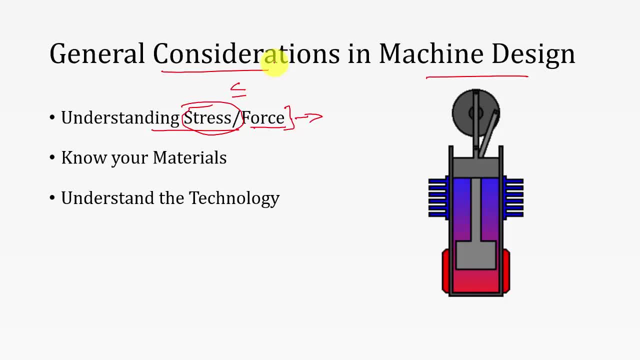 so that is the basic behind this first point. ok, then the second one is: know your material. we have to choose the material based on the load carrying capacity and based on the working environment. ok, so there are. all the materials have some mechanical properties, chemical properties. then, based on all these properties, we have to select a new material, or you have to select. 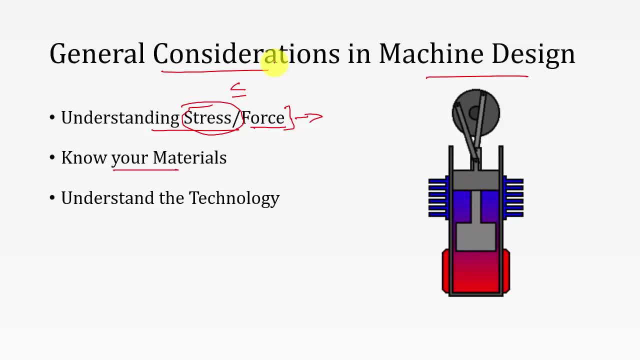 an existing material for your machine element, then understanding the technology. so what is the technology behind that, what is the mechanism behind that, so that we have to identify. so how we are performing the job. for example, here the reciprocating motion of the piston is converted into rotary motion. so how we are going to convert the reciprocating motion. 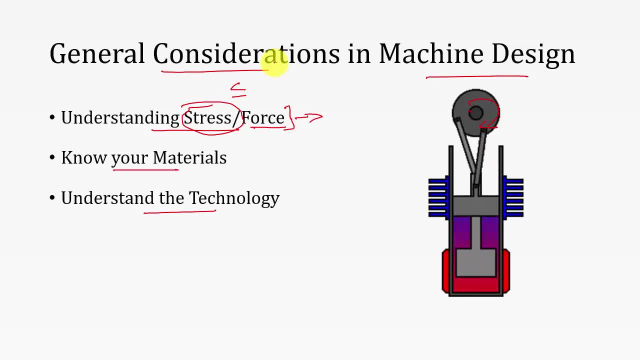 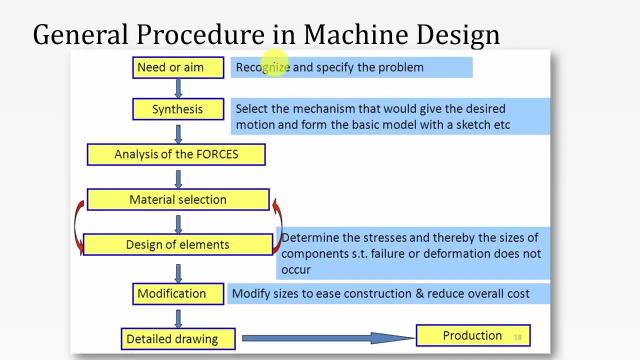 into a rotary motion. there are plenty of mechanisms are available to convert a reciprocating into a rotary motion. so in our application, what type of mechanism we are going to choose? that is the that one. so these three parameters are very important before starting the design. now, this is the general procedure of machine design, so the entire procedure of the design. 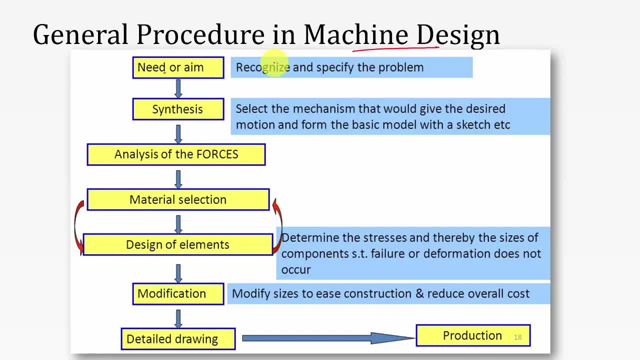 process. so it starts from identification of need, so recognition or specify the problem. so if you are designing a new machine, then you have to get the need and the purpose of designing that machine. if you are going for any adaptive design, then you have to collect the feedback. 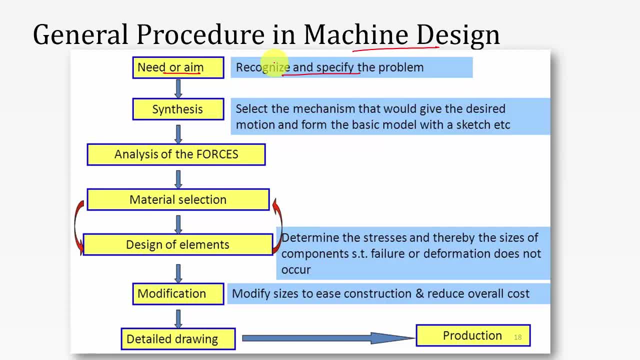 of the customers. so, for example, in the automobile industries generally they will collect feedback from the customers. so after service or after may be five years or ten years of the service of the customer, they will collect the feedback and they will use that feedback as the input for design. 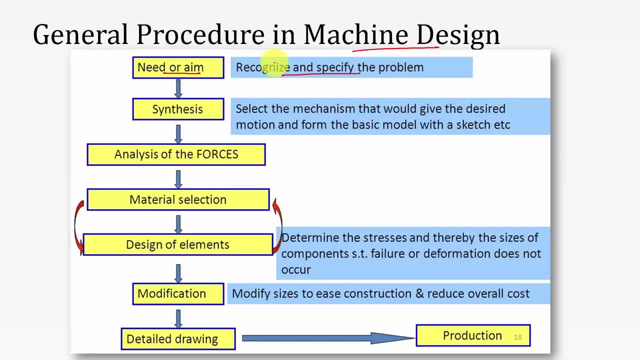 process. so from the feedback they will get some new technologies to be included in the machine and they will consider it as the need then. second one is synthesis. so in the synthesis state we have to select the nature of mechanism that would give the desired motion to form. 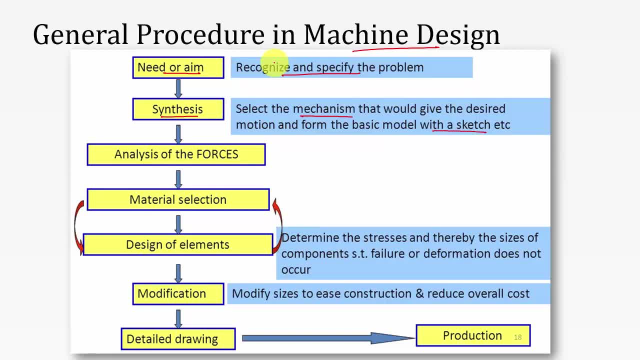 the basic model with a sketch. so here we have to construct a conceptual sketch. so the conceptual drawing will define the nature of mechanism. so it wouldn't give you the detailed dimension but it will give you the nature of mechanism and the types of machine elements you are going to use. 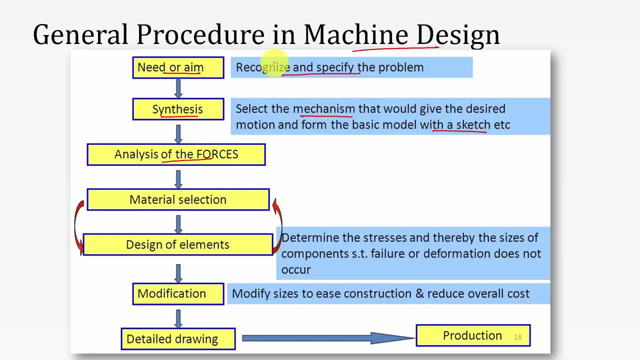 then next one is analysis of forces. so once after finalizing the nature of mechanism, then we can analyze the force, so what type of forces will be acting and what will be the magnitude of that forces. so that kind of analysis you can do it in the third stage. then the fourth stage is material. 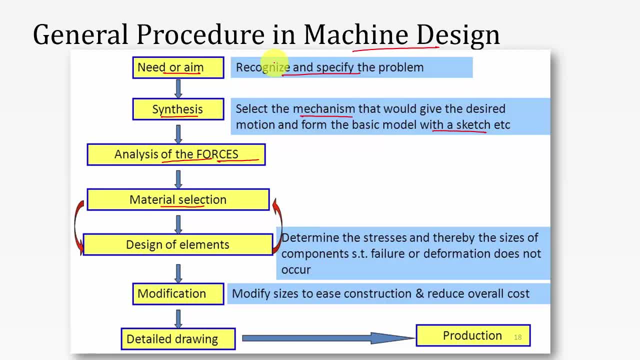 selection. so once after identifying the nature of the force, then we can select the material, because the material selection mainly depends on the nature of force. so if you are having a less amount of force, then you can go for low strength material. so if you are going to, if you need to withstand heavy amount of forces, then you can go for strong materials. 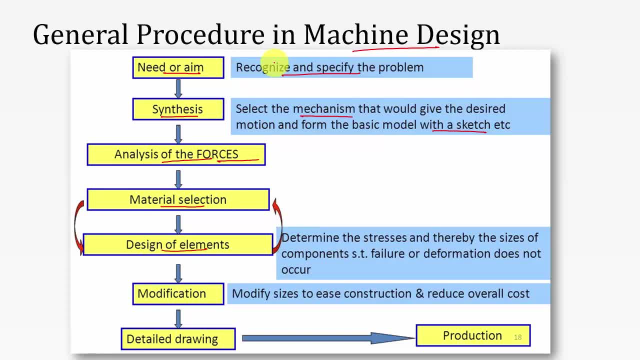 okay, so that is how you have to select the material, then design of the elements. so you have to design the individual elements. so, for example, if you have a shaft, then you have to design the shaft separately. if you have a coupling, then you have to design the. 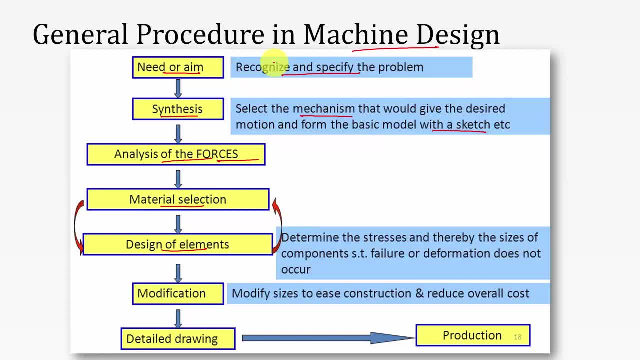 coupling separately. so in during that design, you have to check the safety also. so check the safety means you have to verify whether your design is capable of resisting the forces or not. so if it is not, then you have to change the material or you have to change the dimension. 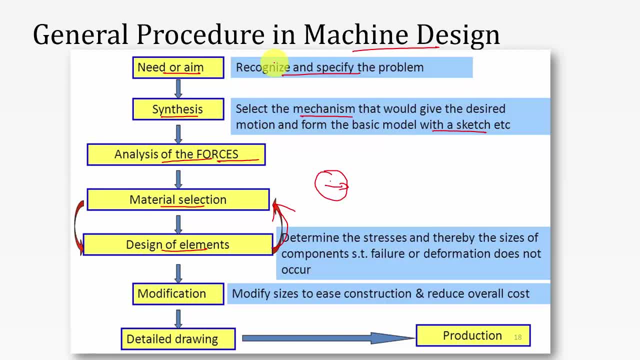 so, for example, I am going to design- I have designed- a shaft of size Z, that is, 40 mm. so I have to check whether the 40 mm shaft is capable of withstanding the loads. so if it is not capable, then we have to increase the size from 40 to 45, or 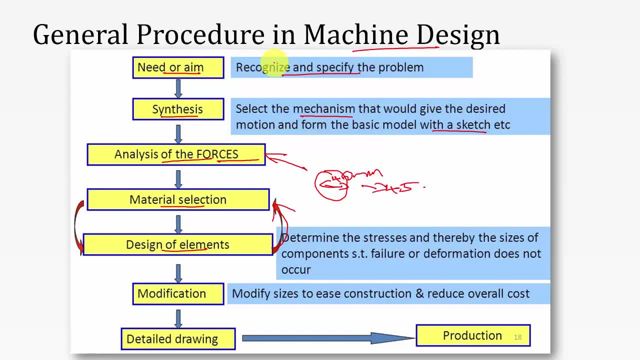 if you have any size constraints, then you can change the material. so instead of a low strength material, then you can go for high strength material, okay, so that is why the material selection and the design of machine elements is interlinked. so I have to check whether the 40 mm shaft is capable of withstanding the loads. so if 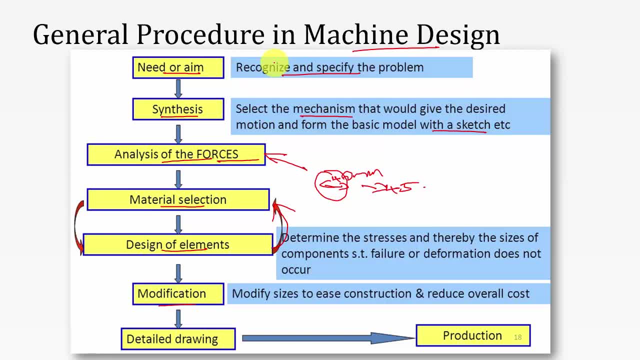 it is not capable, then you can go for high strength material. okay. so that is why the material selection and the design of machine elements is interlinked. so after designing all the machine elements, the next one is modification. so in the modification stage we can change the construction to reduce the overall cost. so here you can do some modifications. 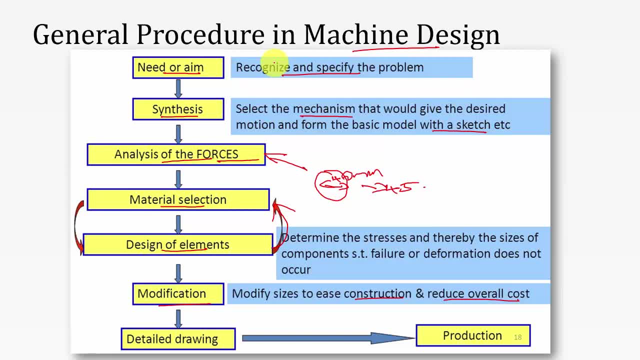 here and there to provide some ergonomics in the machine and to provide some good aesthetics and to improve the quality and to reduce the overall cost. we can do the modification without finished till the end. for further designs on engine details, please watch the process as explained in the Follow. 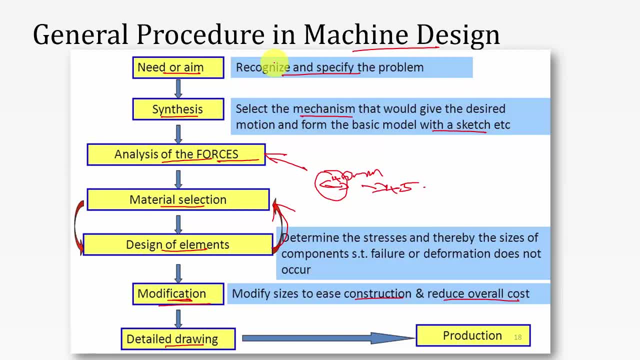 the description box below. so these were the materials we will be using and classifications also given in this tutorial. using Benz engine we will be working with their Mahoban Machinery, which is the öğrencir of Tom vor Conservative beef. So in this process, in our subject, we are going to focus only on this stage, that is, design of elements. 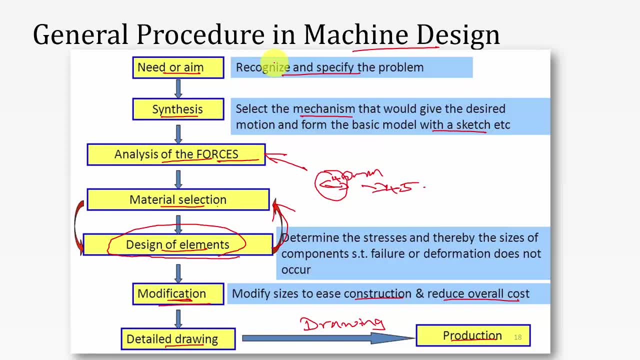 So in the problem they will give you the nature of force acting. You have to select the material and you have to calculate the dimensions of the individual element and you have to check the safety. So if it is not safe then you have to improve the size or otherwise you have to change the material. 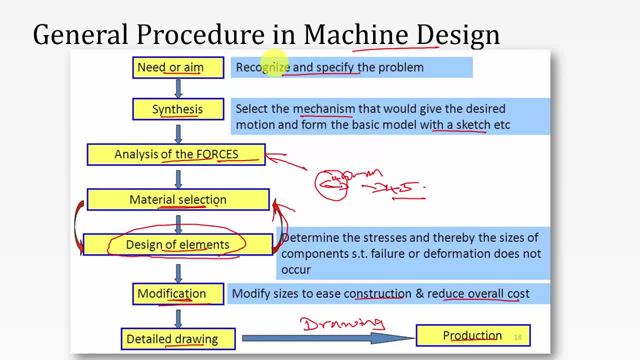 So this part of the design process we are going to deal with in this subject.